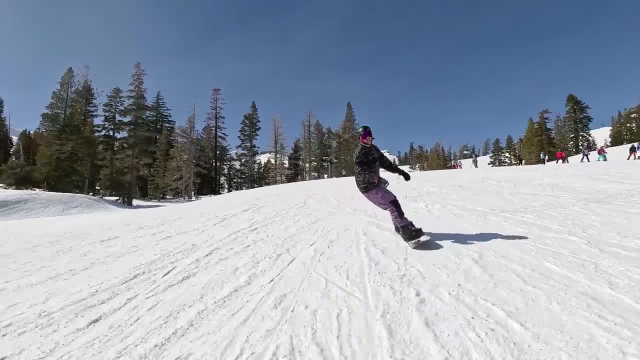 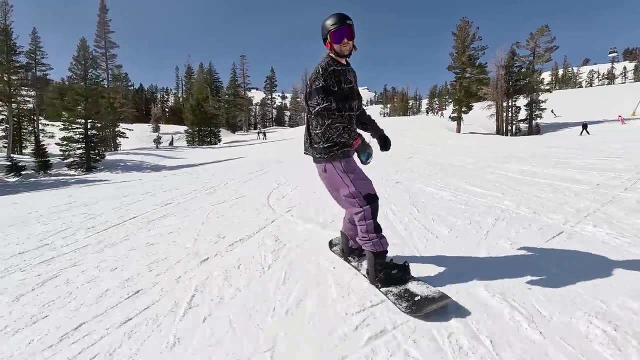 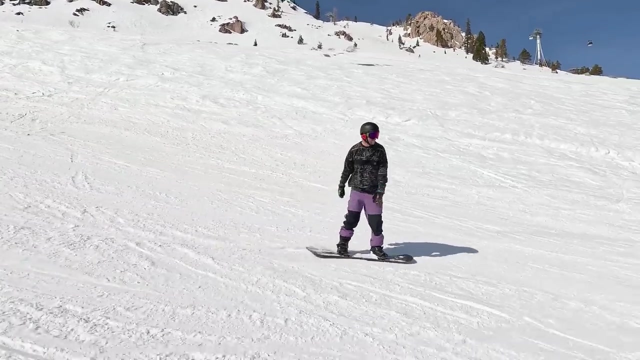 So this is a good habit to get into. So this is a good habit to get into on mellow terrain like this. but as you start to get into more advanced terrain, having your front shoulder to anticipate each turn will really come in handy. So for my heel turn I open up. for my toe turn, I close, and by just constantly having that front, 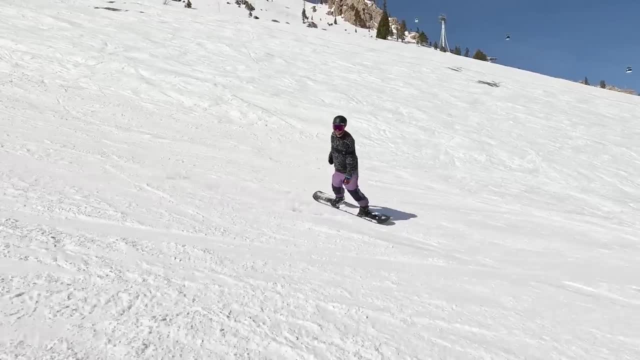 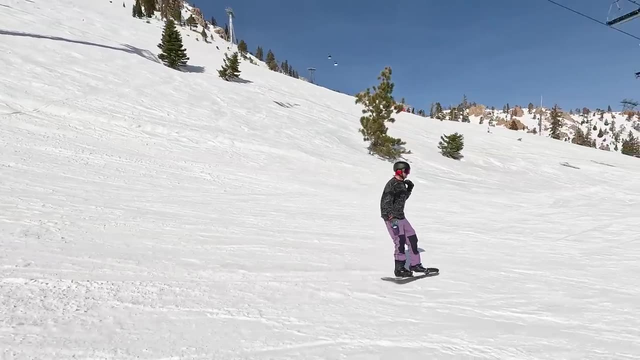 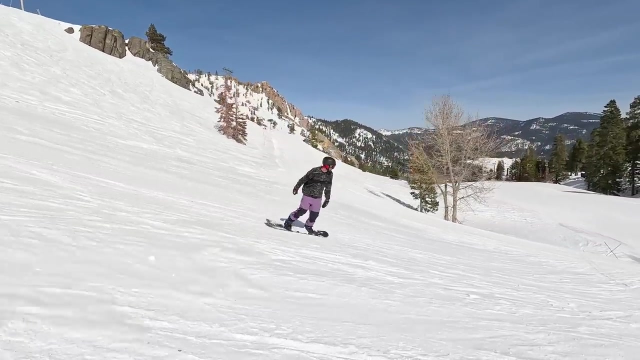 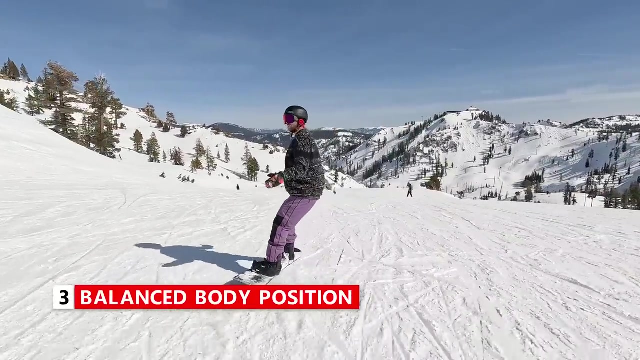 shoulder kind of guide me through each turn. it helps me to initiate the turn and also prevents me from like over steering each turn, because this front shoulder is starting to tell me where to go for my next turn. So experiment using your front shoulder. So another habit to get into is riding with a really balanced body position over top your snowboard, so knees. 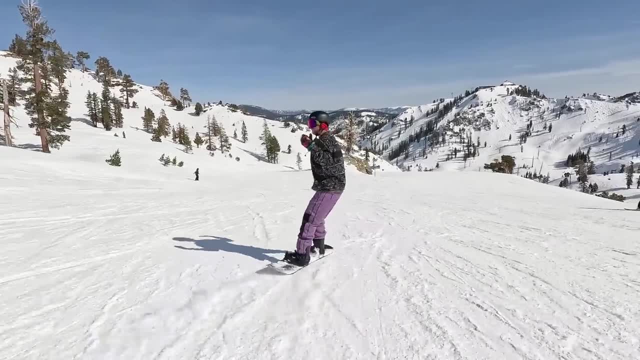 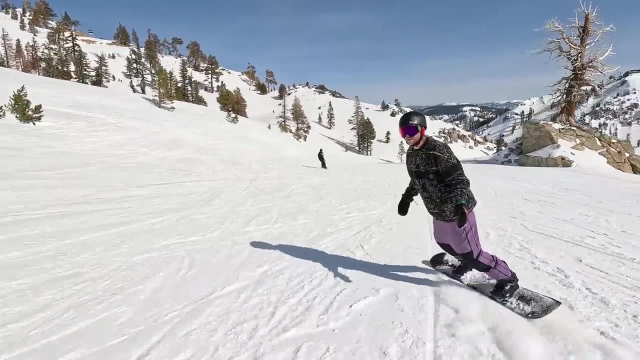 bent, bent at the waist a little bit, but with your back straight and having this balanced body position. it just allows you to keep your weight on top of your board so that when you get onto your edges, your edges don't slide out. It's when you put your weight out past. 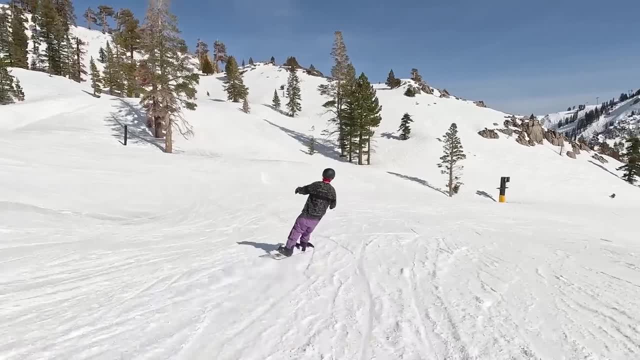 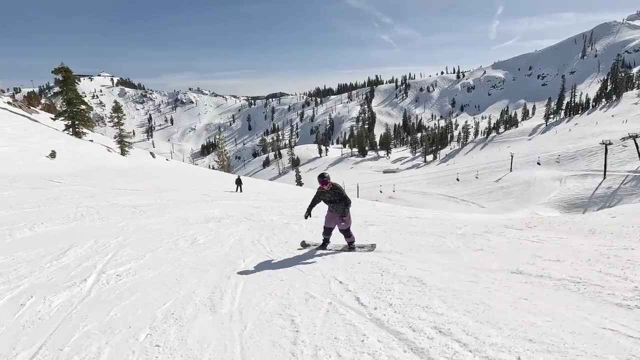 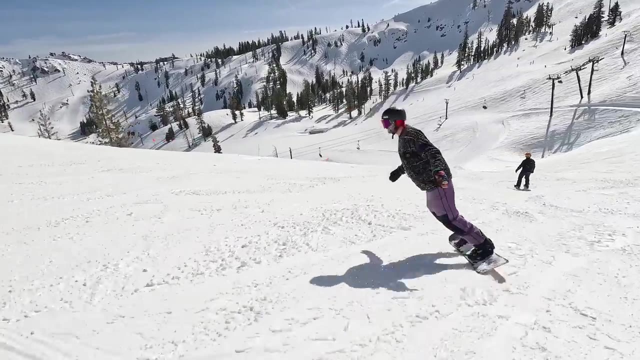 Your edge edge. so, for example, on your heels. if you're too far back, your heel is going to start to chatter. or if you're bent over too much on your toes, that's when your toe edge can start to like chatter as well. So, having your knees bent- a balanced body position- this just puts you into. 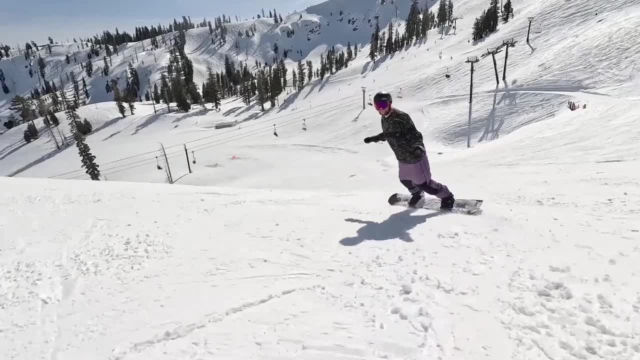 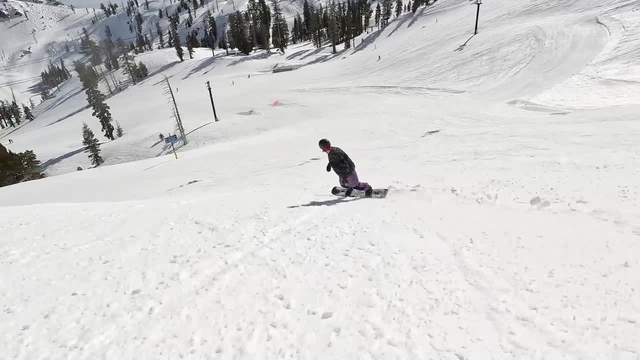 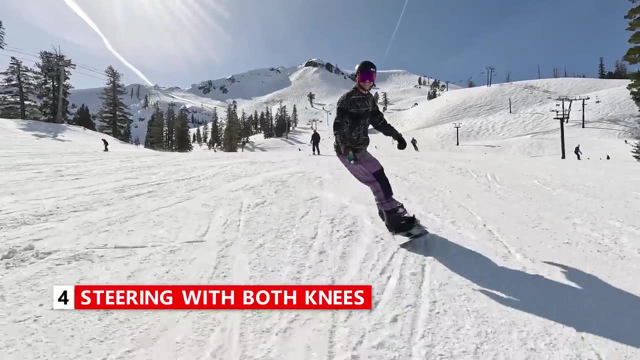 that spot where your weight's over top of your board, you're going to feel in control with your edges and you can really handle anything that the run throws at you. Another good habit to get into is steering with each knee independently. So by steering with your knees it's really going to. 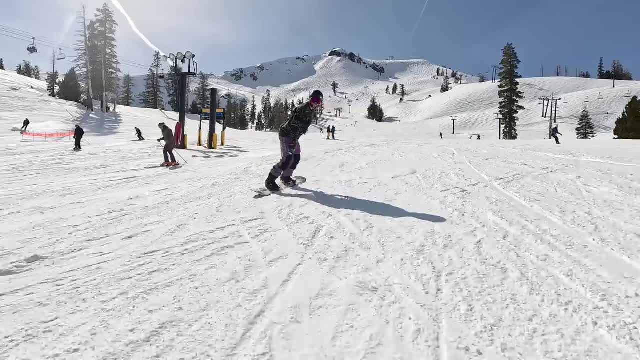 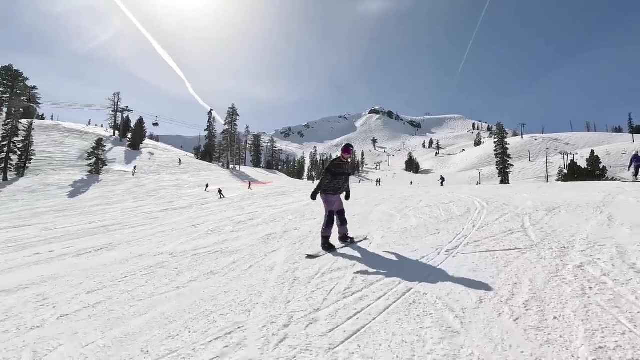 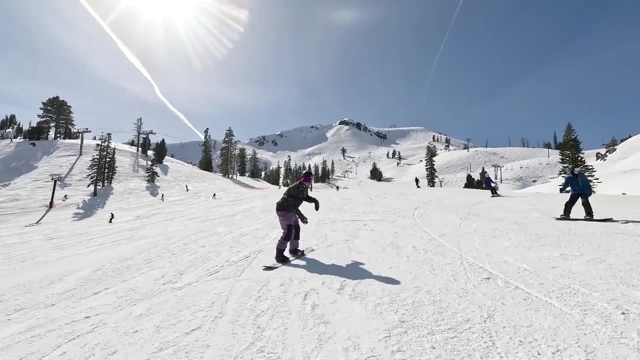 allow you to steer your snowboard much more aggressively. So when you first start out snowboarding, you learn to use that front knee and you open up that front knee for the heel, close it for the toe. but once you start adding in your back knee as well, then your turns become like much more dynamic. 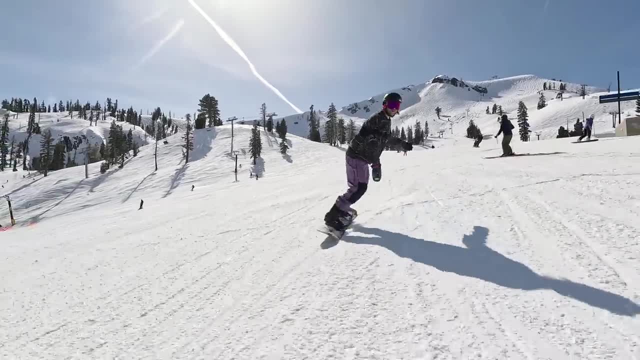 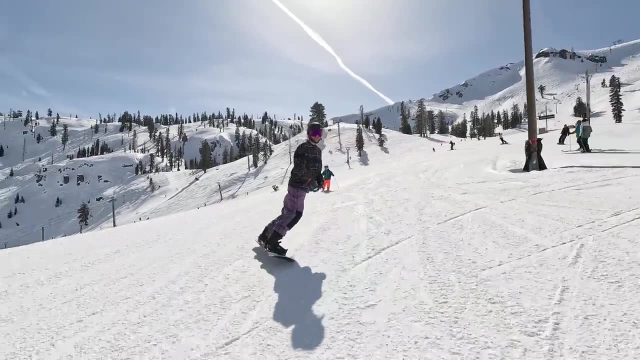 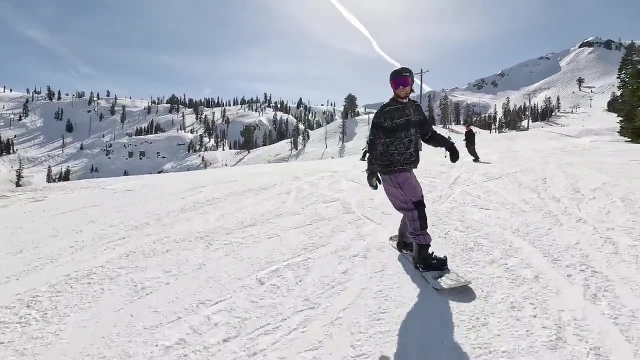 and like right now. this is a lot of work, but if I was in some terrain where I had to do some quick turns, using both knees to steer comes in really handy. So get in the habit of steering with your front knee first, then, when that feels comfortable, add in the back knee. practice it. 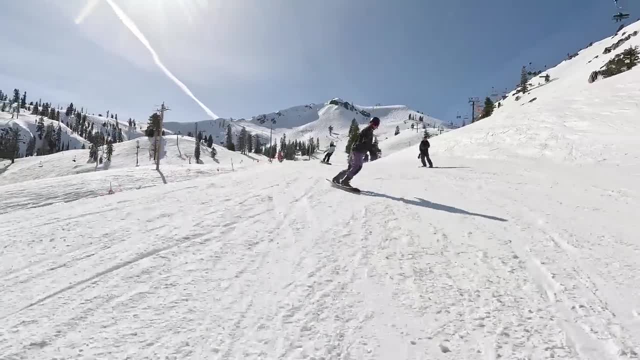 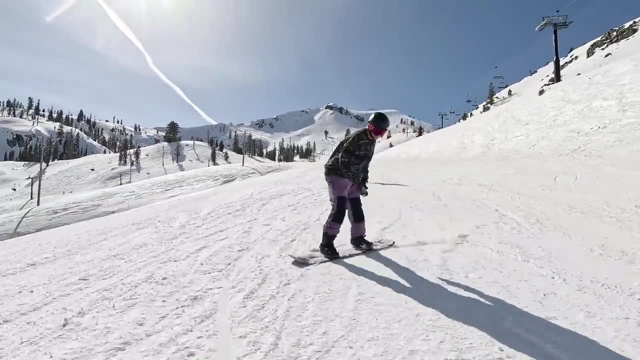 someplace that's mellow and then, when you're done, you can start adding in your back knee and when you get to that more difficult terrain you're really going to feel the steering capabilities of having both knees really comes in useful. The next habit to get into is starting to play around with your weight and getting your 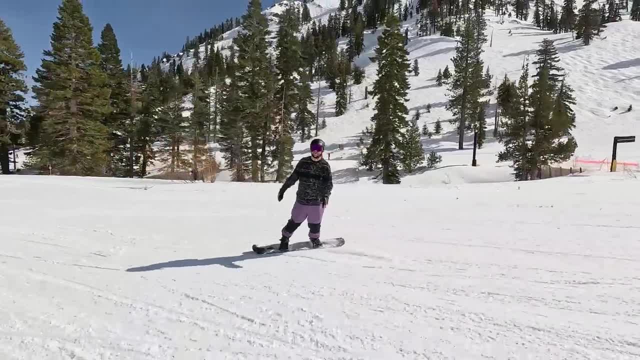 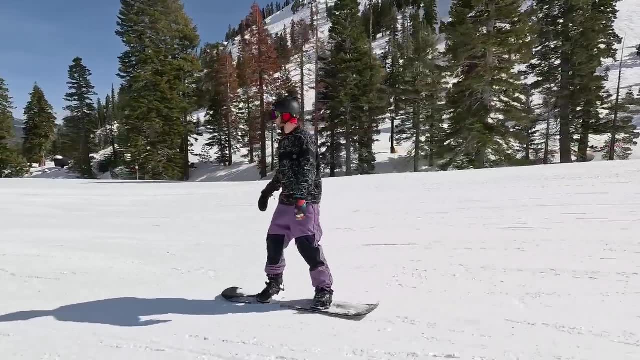 weight more forward towards your nose or more back towards your tail. When you first start out snowboarding, your weight is more or less going to be about centered. but as your turns become more advanced, then that's when you want to have either your weight forward or 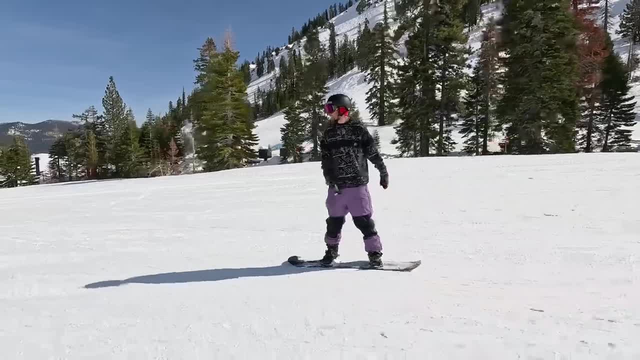 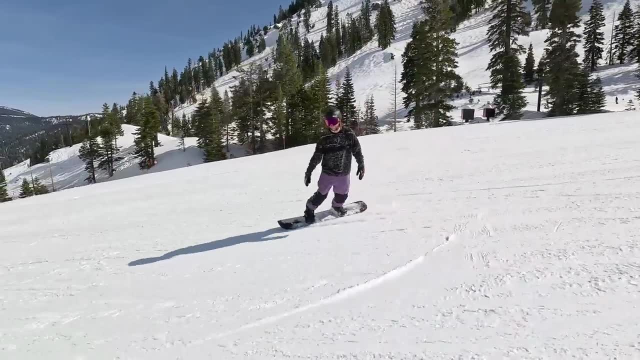 back. This is really going to help make your turns more dynamic. So the times when you want to have your weight more forward is when you're starting a turn. So to start a turn, having a bit more weight onto your front foot really comes in handy. It gets your weight down the 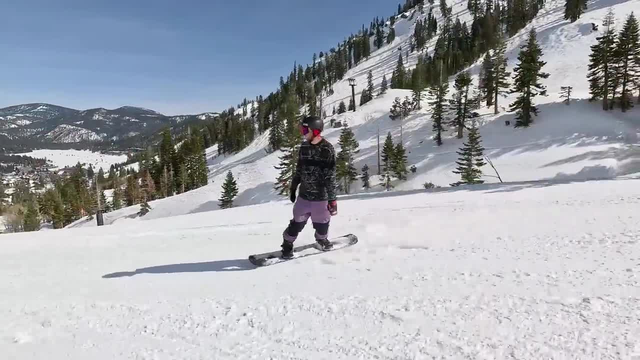 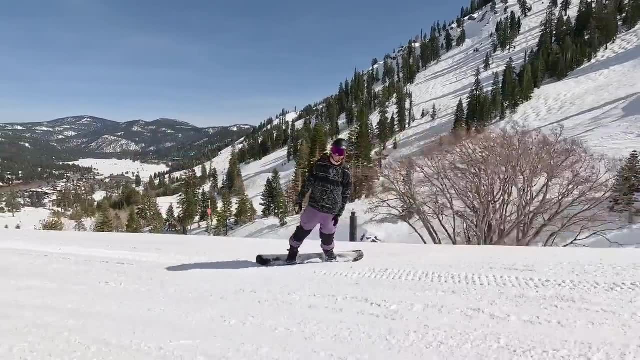 hill and helps you to initiate that turn. And then where you want to have your weight more back is, as a turn comes around towards the end of a turn. So getting your weight more into your back foot really helps you to hold that edge and just keeps your edge. 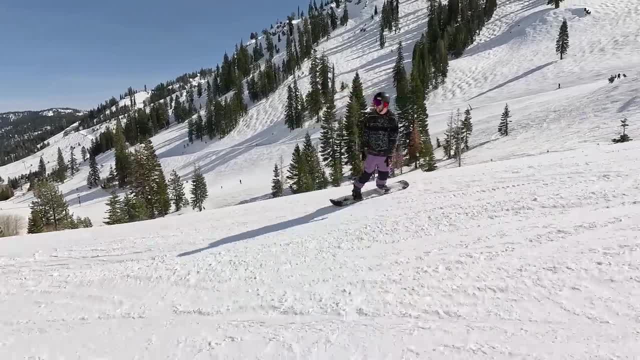 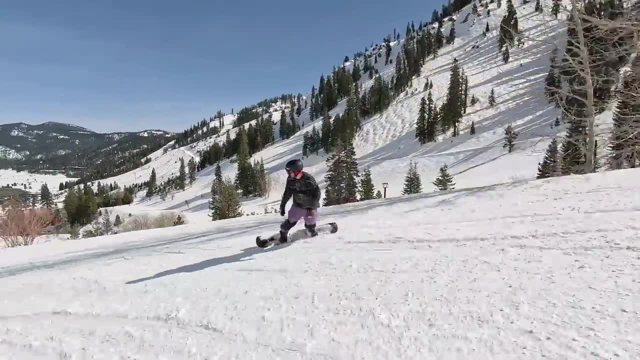 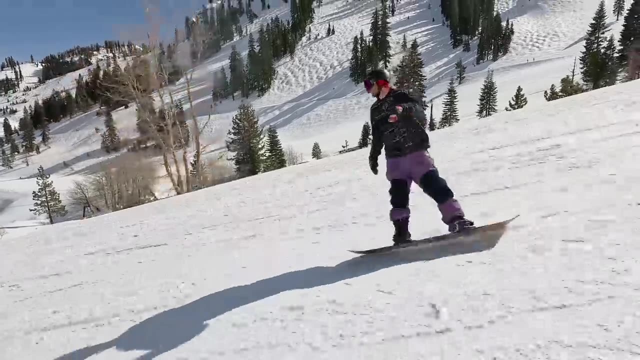 more in contact with the snow. So down here let's do a few. So I start out forward, come around back, start out forward, come around back, and just constantly alternating that weight between my front and back foot, I think you're going to notice that your edge stays in more contact with the snow you have. 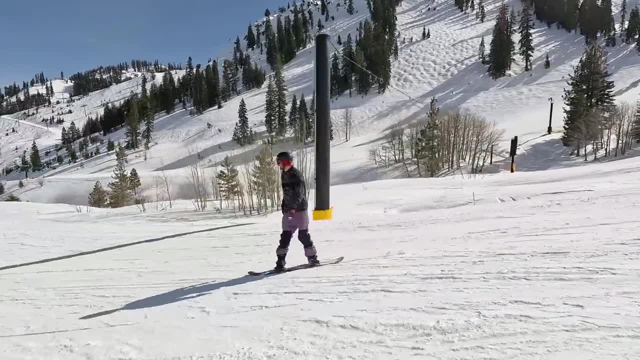 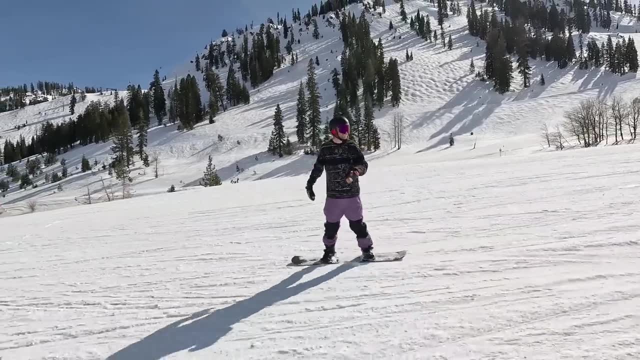 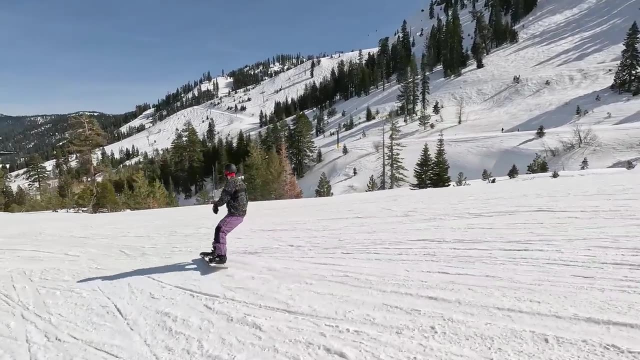 more control and it's easier to initiate that turn. It can be mellow and you can get away with having equal weight on super easy runs, but when you get to a really steep pitch, having your weight forward and then back is really going to come in handy. 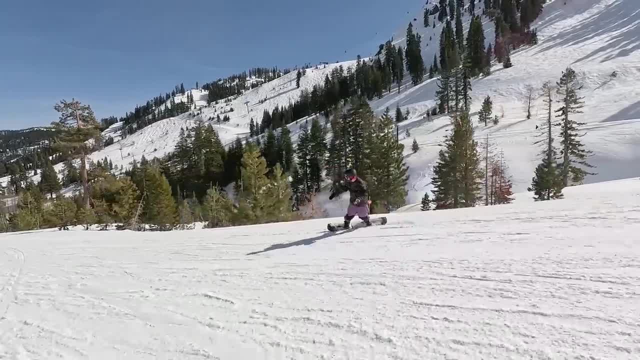 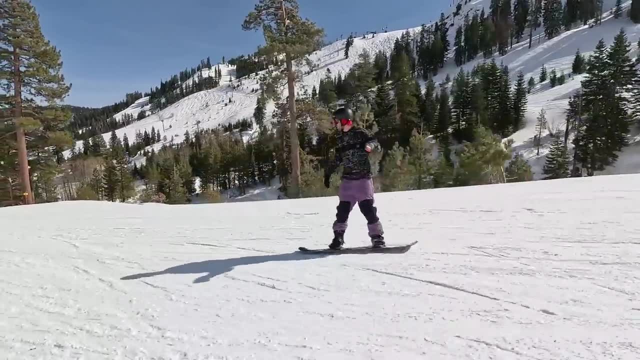 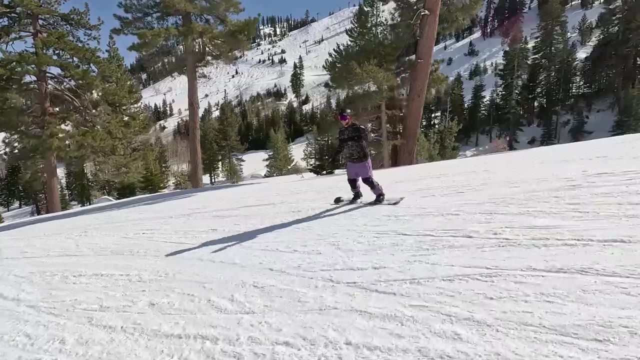 So on this run I'm just playing around with my weight, feeling it out. To me, the feeling of having my weight on my back foot as a turn comes around feels super good, And just alternating it constantly. It takes a bit of practice, but once you get into that habit you're going to find yourself. 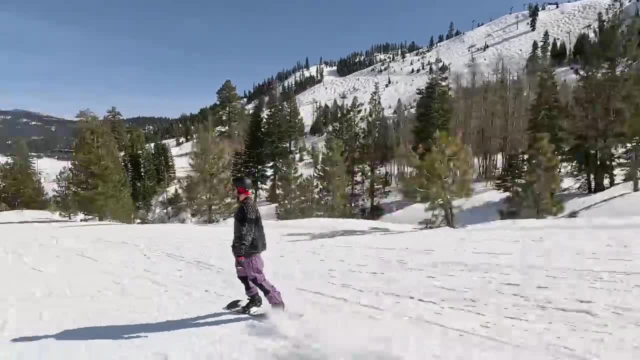 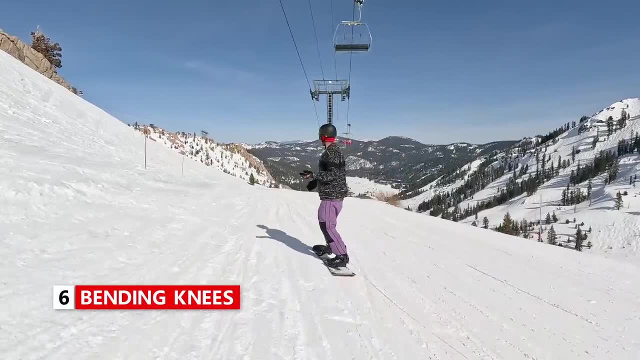 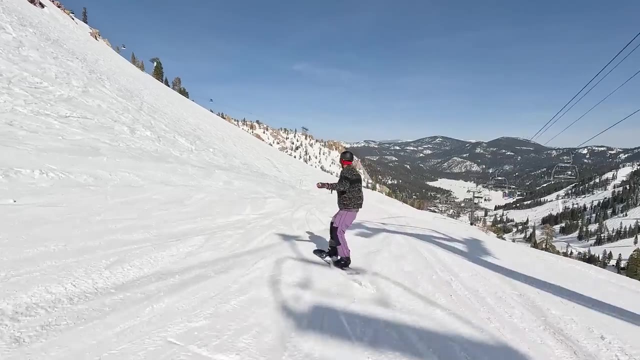 doing it all the time through your turns. So a habit that will help you across all your turns is bending your knees and really using them like shock absorbers. So by bending your knees, you're going to get lower to the snow, so lowering your center of gravity, which will give you better balance. But also, if you come, 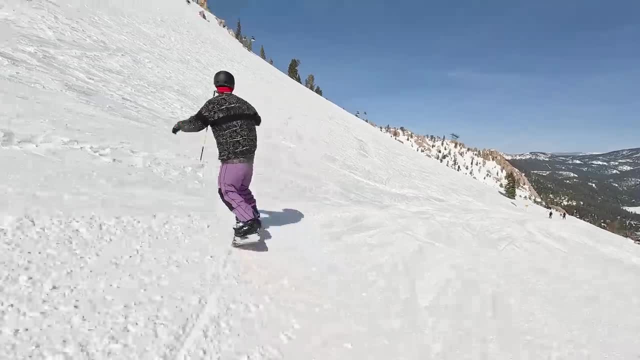 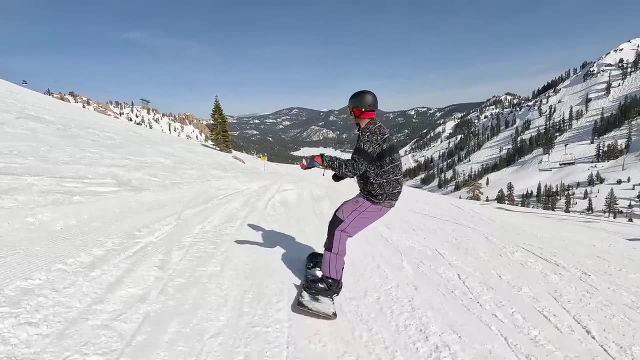 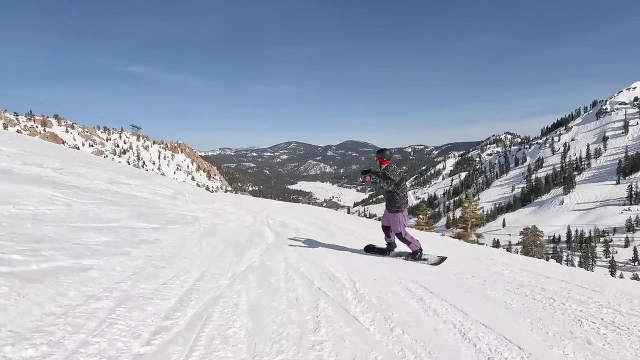 across any bumps in the snow, like riding up the side. using your knees can help you to absorb all of that. keep your snowboard in constant contact with the snow and give you more control So, as you ride, be aware of how much you're bending your knees. You can even think about. 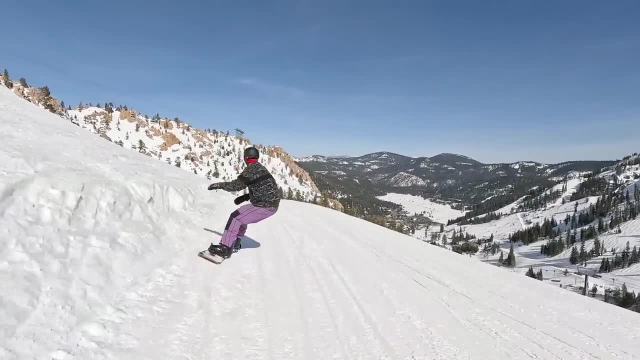 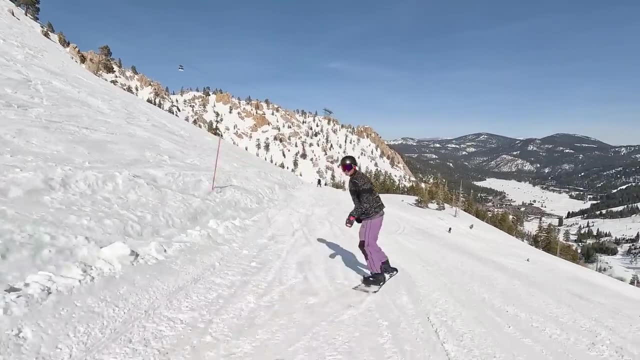 bending your knees through each turn, so like up and down. This helps you to absorb the pressure that builds on your snowboard, And bending your knees up the side And just overall having that lower center of gravity, will improve your snowboarding. Having your knees bent will also. 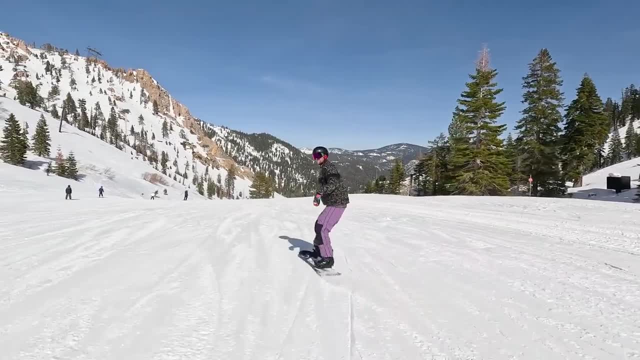 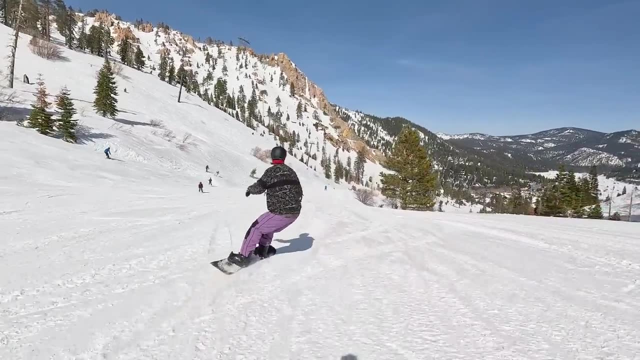 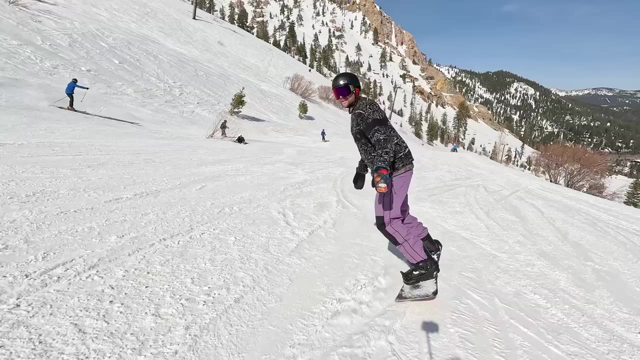 help you to steer your snowboard better, keeping your knees a bit more free with them bent, And then also just helps you to absorb the pressure that gets built up on your snowboard So as each turn comes around, you can bend down, absorb that pressure and keep your snowboard. 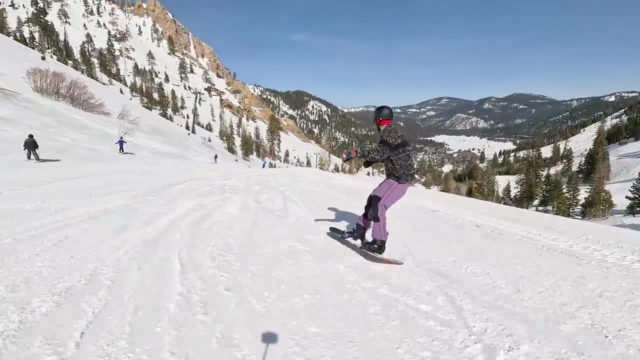 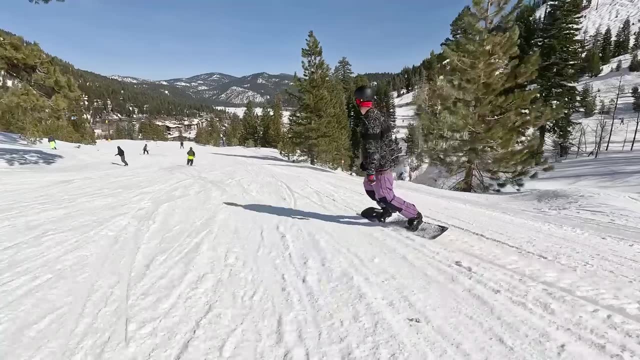 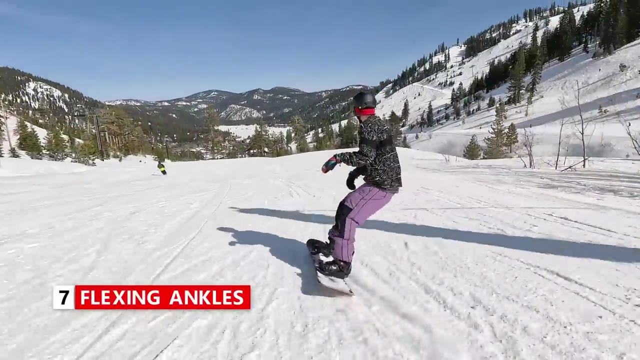 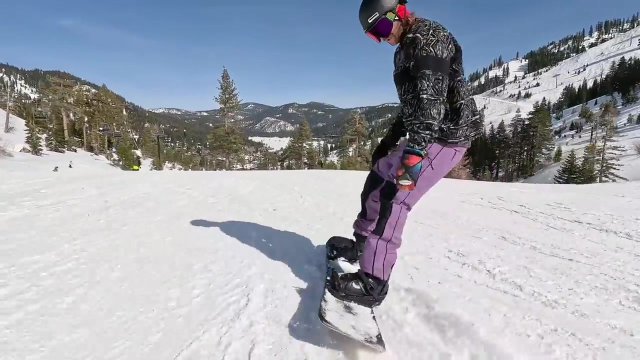 in constant contact with the snow. So in so many different ways bending your knees just helps to overall improve your riding. So another habit to get into is starting to flex your ankles to really start to get your board more onto edge, So not only for carving but just for your turns in general. 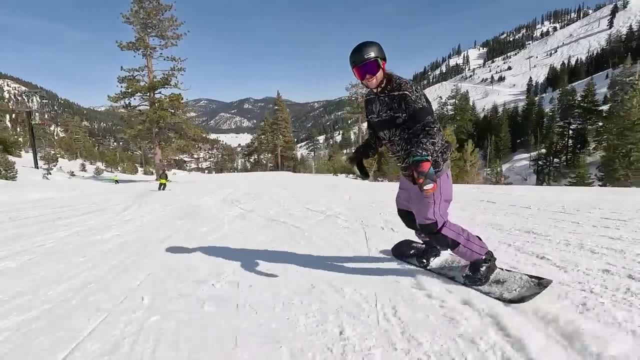 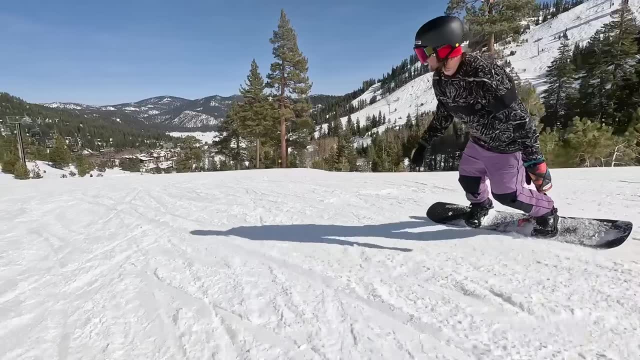 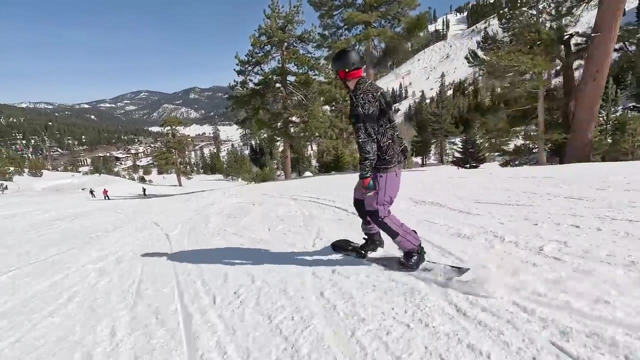 Really starting to be aware of your edges and use your ankles to flex and get your snowboard more on edge and more onto your edge to get into a carving turn By being aware of your ankles can allow you to be more maneuverable with your snowboard, cut more speed and, just overall, be in. 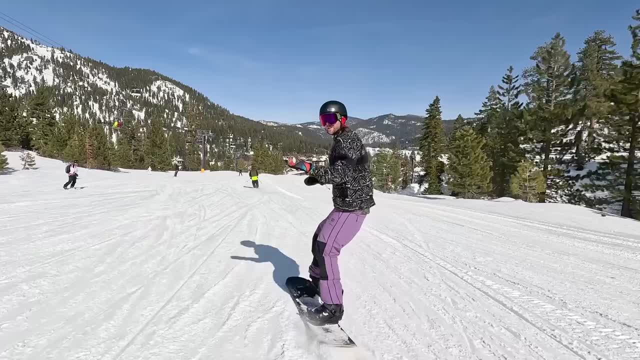 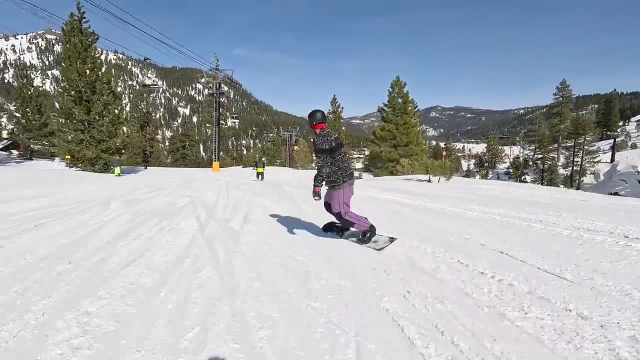 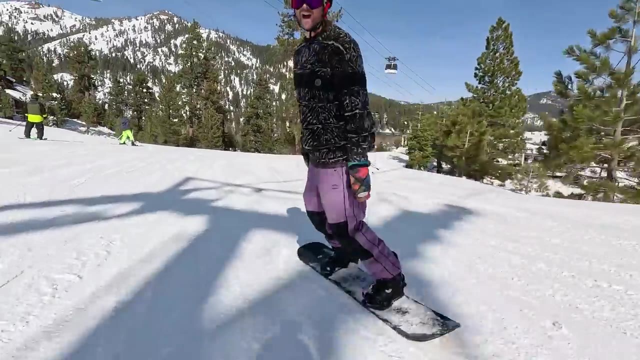 more control By playing around with how much you let your snowboard get onto edge and how much you use your ankles is really going to determine, like, how much snow you can spray, how much speed you can control and also how well you can carve. So play around with your ankle movements and it's 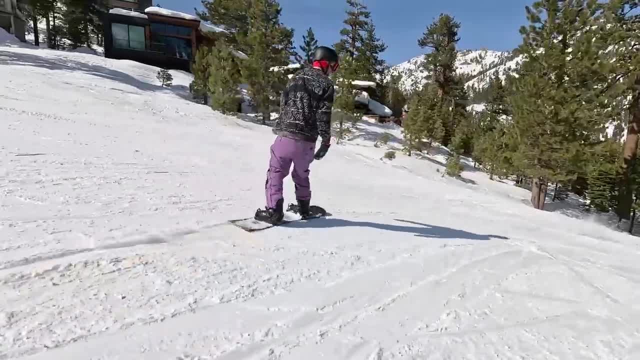 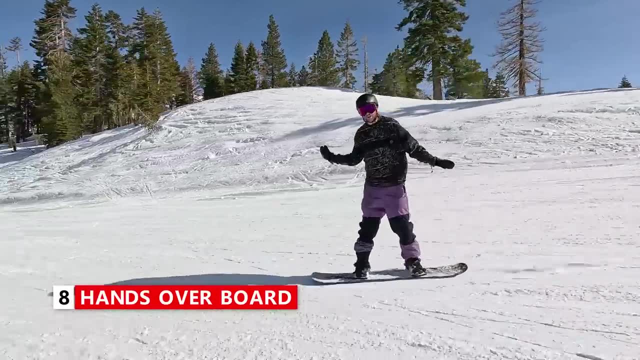 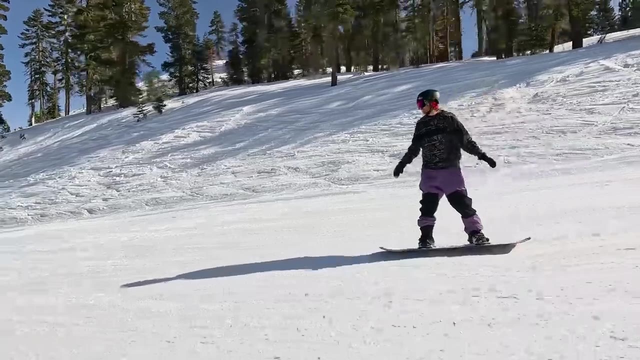 really going to open up a lot of different things in your riding. Another really good habit to get into is to ride with your hands over top of your board and looking over top of your shoulder. This is another balanced position that you can get in the habit of doing and just overall it helps to 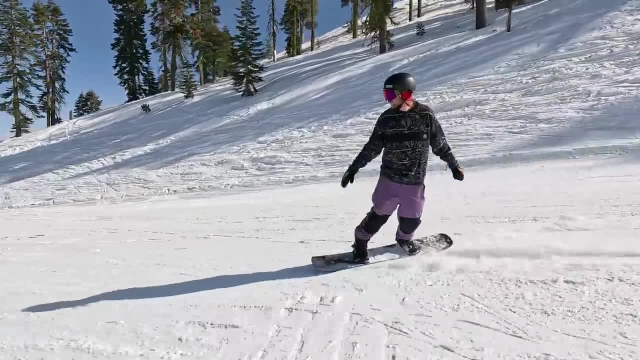 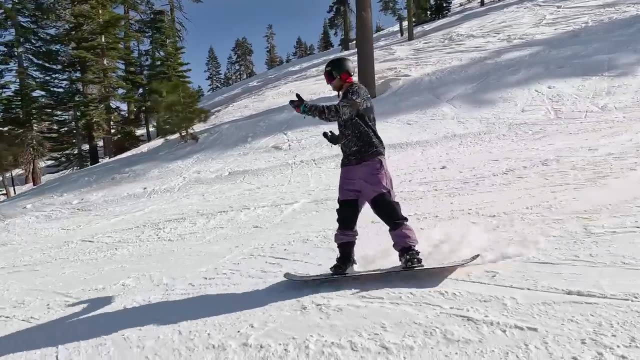 like, keep your turns a bit more. even your balance of your board will be better. and this fix is kind of like a bad habit that can come up is where if you are facing too much of your body down the hill, then you're on your heels a little bit too much. 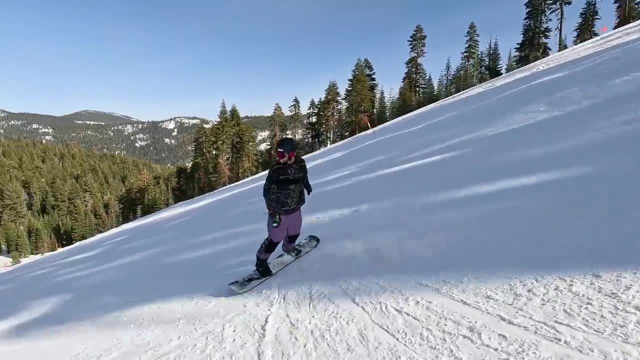 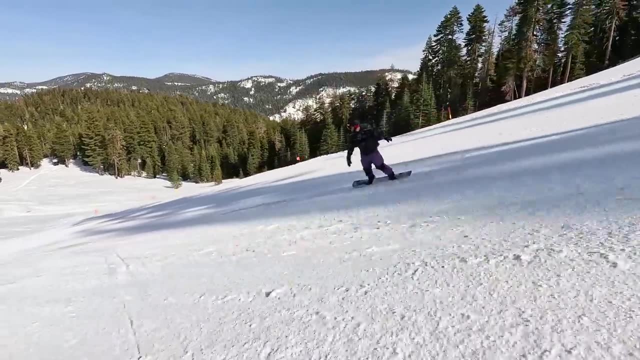 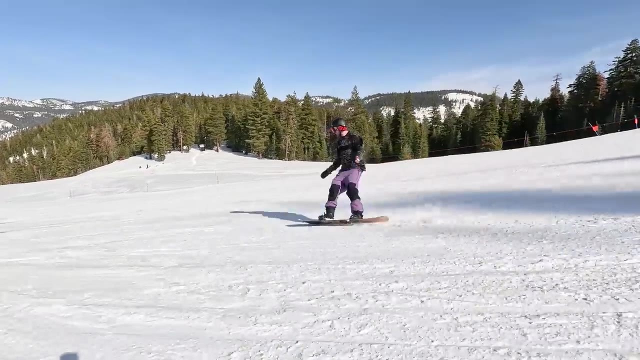 So by making sure your back hand is over your tail and you're looking over your shoulder, it gets you into that habit of committing more to toe turns and it's just going to give you better overall balance, especially when you get to some more difficult terrain Having 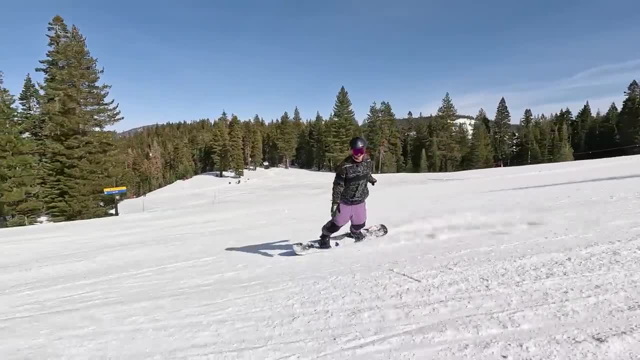 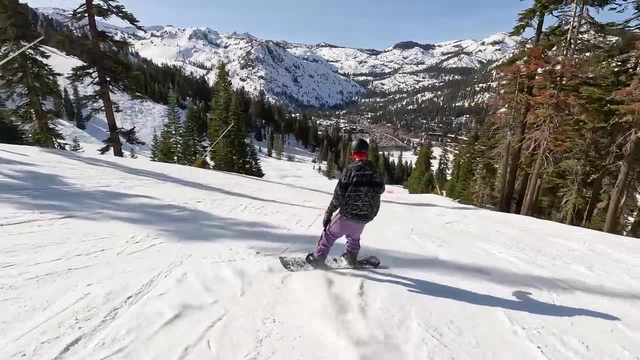 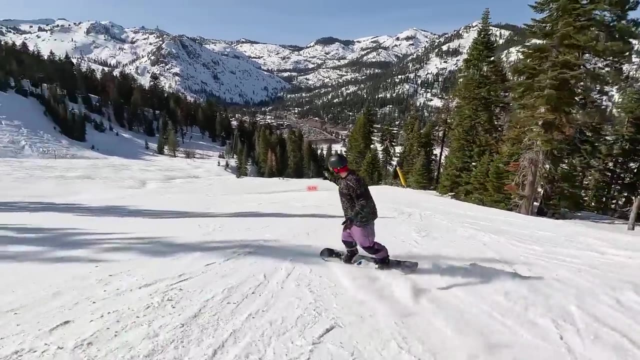 this back hand over your tail really helps you commit more to the toe turn. So another really good habit to get into is looking down the slope and finding all the areas where you want to slow down, where you want to pick up speed and just like scanning ahead. so 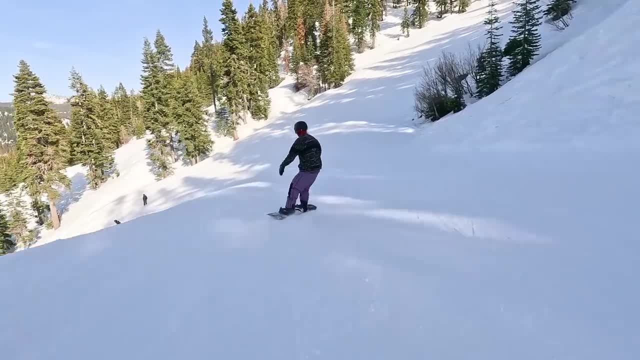 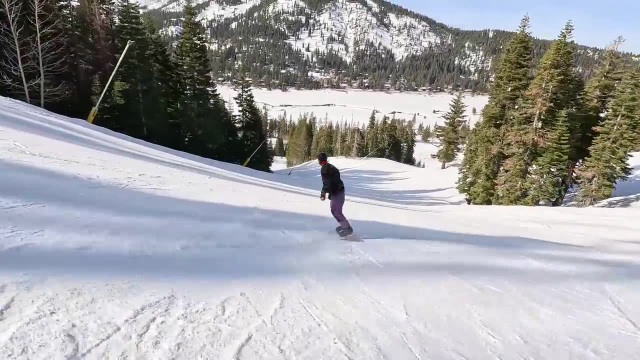 that you know what's coming. The more that you can look ahead, the more confidence it's going to give you. because if you see like a bump ahead, you'll know that's where you need to avoid or slow down. If you see a flat part, that's where you know you need to speed up. 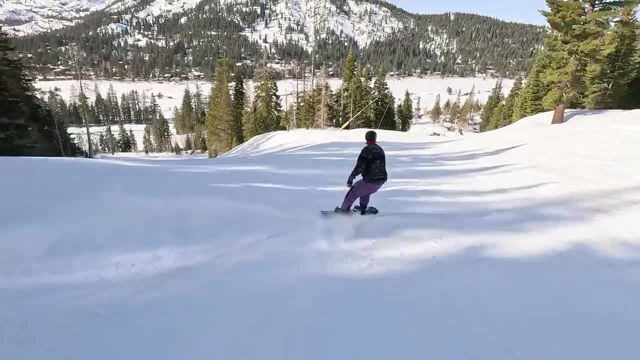 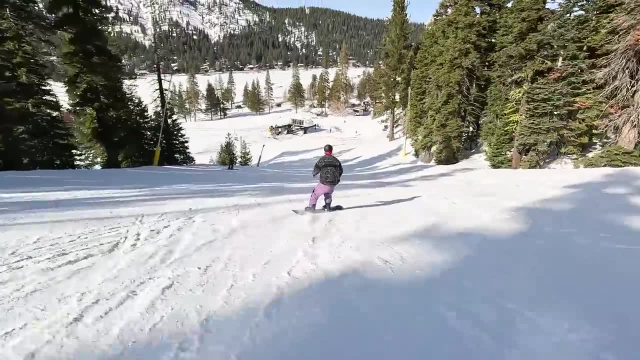 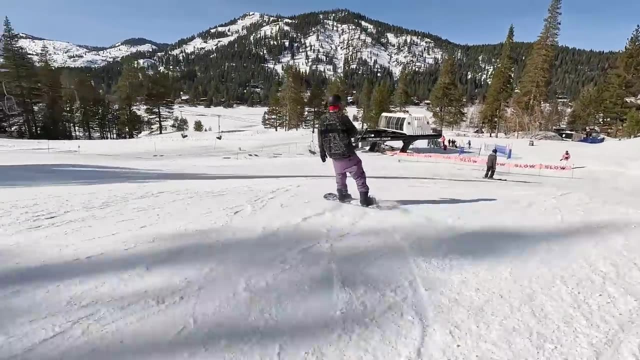 And just by looking ahead and scanning the terrain, it's going to give you a lot of confidence to ride with more control and it'll just, in general, improve your riding because you'll be able to anticipate anything that the run throws at you. Oh, like I'm looking ahead and there's a little. 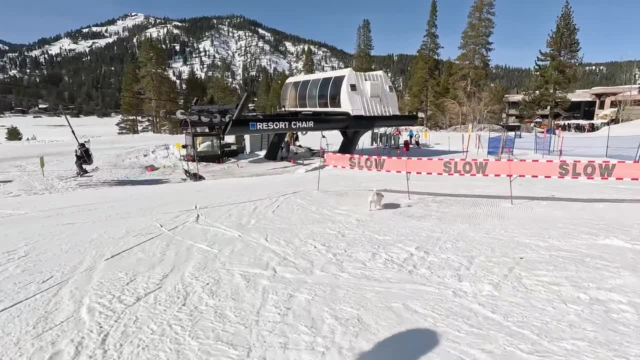 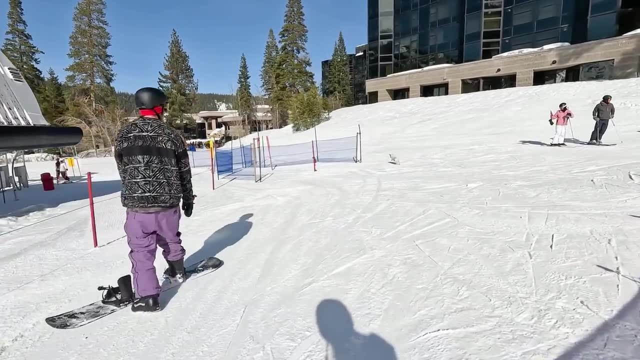 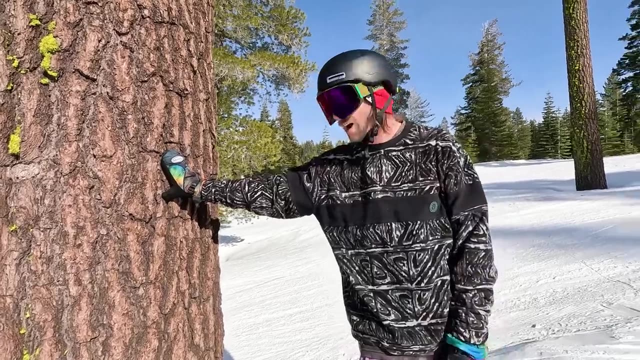 Poochie, Hey, buddy. Oh, let's go for a pee. Amazing guys. so I hope those habits will help improve your snowboarding. If you have any questions, let me know. down below in the description I'm also doing a camp this summer with the High Cascade, If you want to. 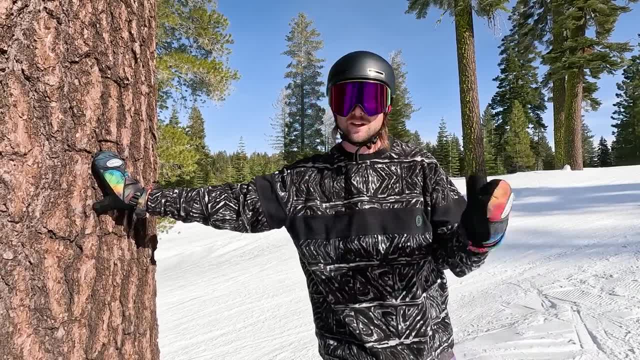 come snowboard with me this summer. I'll put a link to that below. Also, subscribe here to Snowboard Pro Camp. be safe out there, have fun progressing with your riding and I'll see you in the next video.